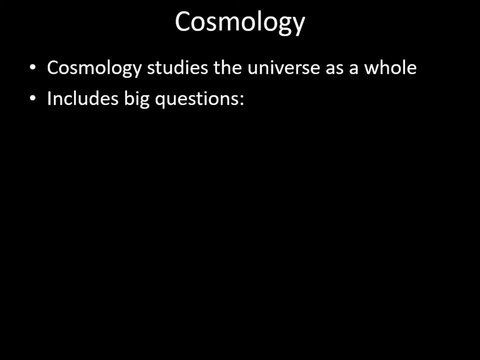 This is the branch of science that tackles the really big questions. Some of these include: how did the universe form and how has it evolved since its formation? What is the eventual fate of the universe universe? How did the large-scale structures, such as clusters and superclusters of galaxies and the 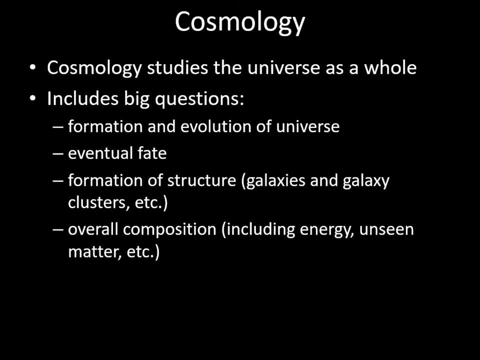 voids between them form? What is the overall composition of the universe, and how did this come about? Cosmologists don't have all of the answers to these questions today, but the fact that we can even begin to address questions like this in a scientific way is an indication of just 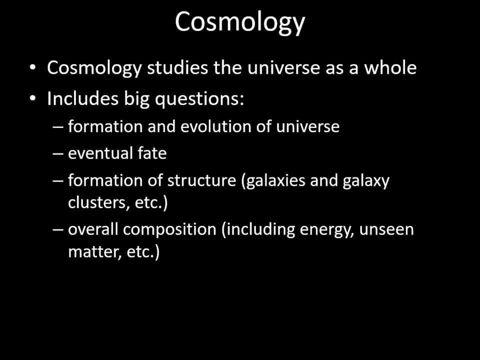 how far our understanding of the universe and the processes that operate in it has developed in the last two centuries. It was theoretical developments like the laws of energy in the 19th century and relativity and quantum mechanics in the early 20th century, along with observations like the 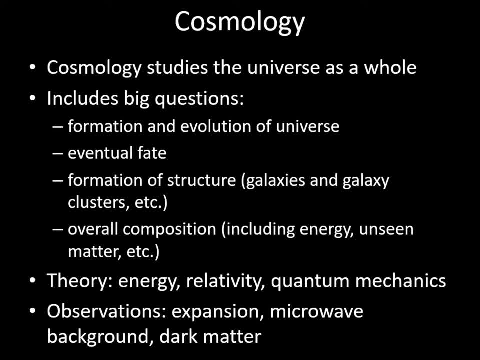 expansion of the universe in the early 20th century, the cosmic microwave background in the middle of the 20th century and the evidence for dark matter in the late 20th century that have allowed the development of a scientific model of the universe and its evolution. 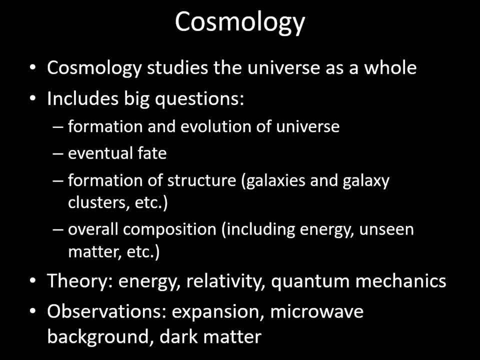 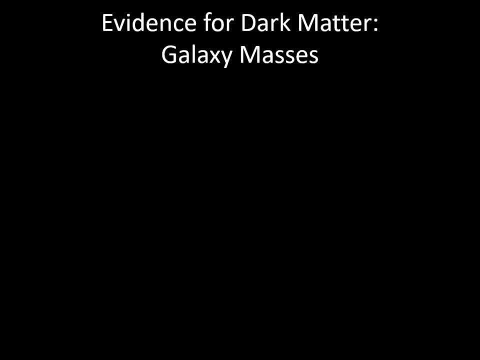 So let's start our look at the universe as a whole by asking a question that should be easy, but isn't. What is the universe made of? As we've mentioned earlier, we can use orbits to measure masses. We've seen how the orbits of binary stars around each 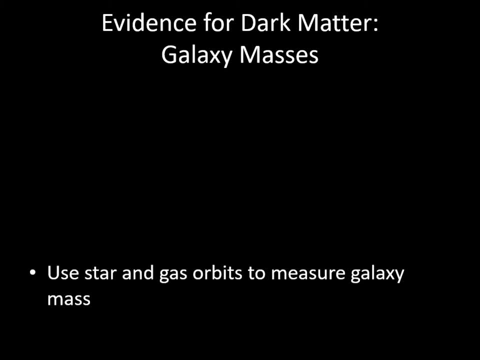 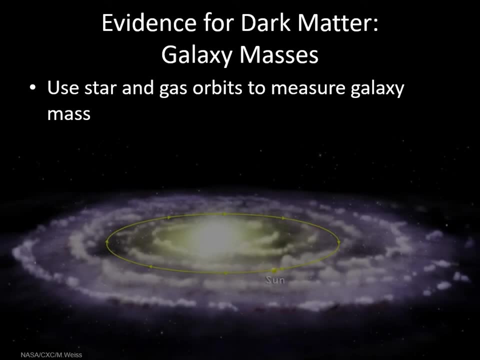 other can be used to find the masses of stars. The same principle can also be applied to stars in gas orbiting around a galaxy. If we measure the star'sastre, this in a way horizontal frequency, denotes the mass of the galaxy, which we call the relative mass. Soёn we created a call on 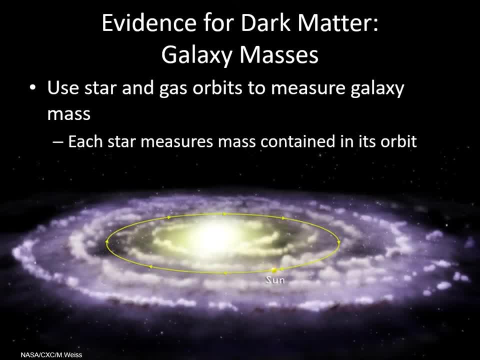 speed of a star in a galaxy, we get a good estimate of the mass of the galaxy enclosed by that star's orbit. For example, the yellow curve in the diagram below shows the orbit of the Sun around the Milky Way. The Sun's orbit speed in the galaxy tells us how much. 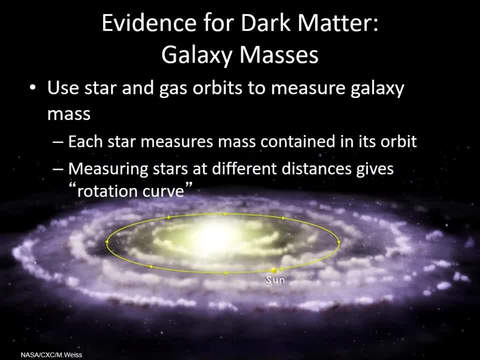 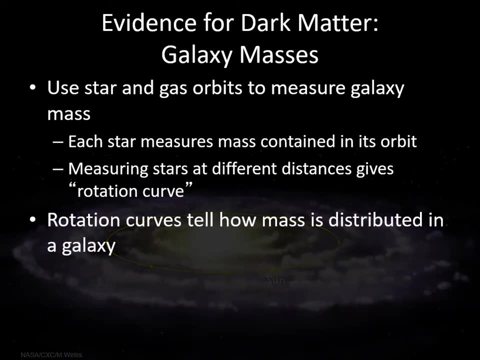 mass is within this orbit. By measuring the orbit speeds of stars in different parts of a galaxy, we can make a graph showing the orbit speed at different distances from the center of the galaxy. This is called a rotation curve and it can be used to see how mass 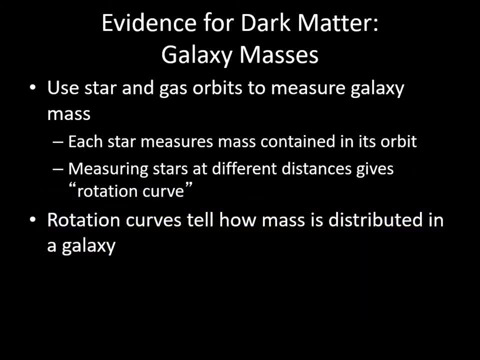 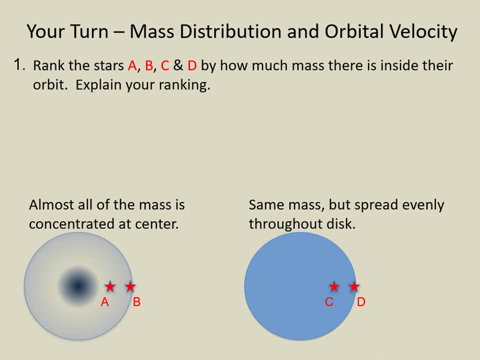 is distributed throughout the galaxy. These two exercises should help you see more specifically how this works. The blue circles represent face-on views of the disk of a spiral galaxy, showing two possible ways the matter might be distributed: Almost all the matter might be concentrated near the center, or the matter might be spread. 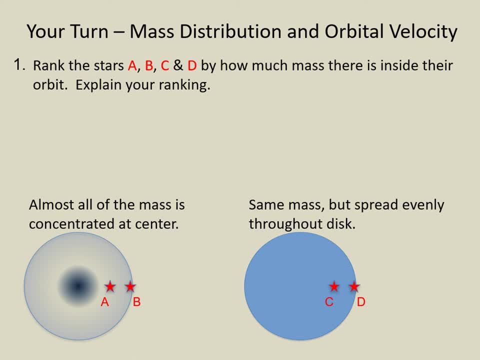 evenly throughout the disk. The letters represent stars that follow approximately circular orbits within the disk. To start with, put the stars in order of how much mass is enclosed within their orbits, from the most to the least amount of mass. There may be two or more stars with. 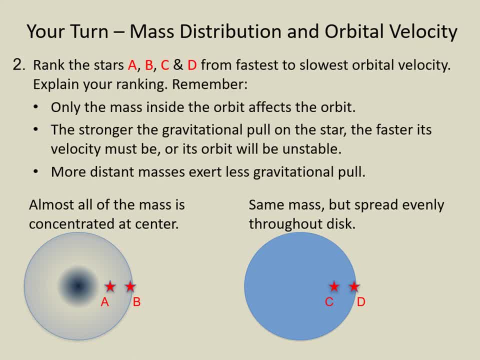 the same amount of mass enclosed. Now that you know how much mass is enclosed in these orbits, the next step is to rank the stars from fastest to slowest velocity. Remember: only the mass inside the orbit affects the orbit. The stronger the gravitational pull on the star, the faster its velocity. 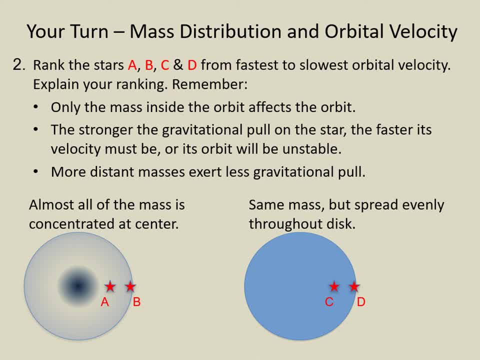 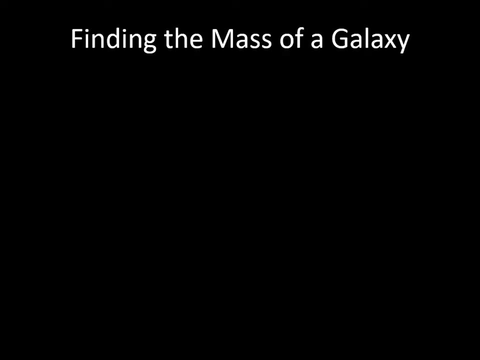 must be, or its orbit will be unstable. Distance matters too, because more distant masses exert less gravitational pull. In fact, we see the effect of distance in our solar system. The most distant planets orbit more slowly. Let's take this discussion a step further and see how we measure the mass of a galaxy. 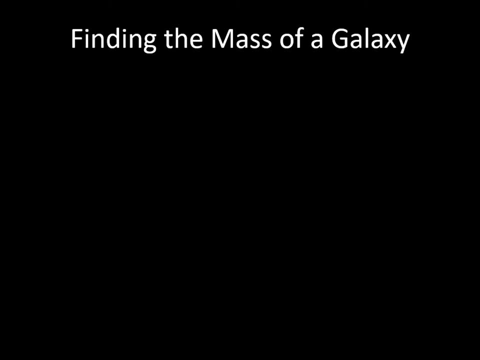 using the orbits of the stars and gas within it. Back in the chapter on motion and energy, we saw that Isaac Newton took Kepler's Third Law of Planetary Motion and updated it so that it could be used to calculate masses. in astronomy, The version we saw for planets was the third law of planetary motion, and 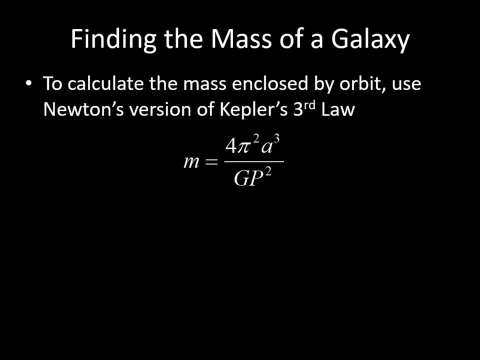 the second law of planetary motion was the third law of planetary motion and the third law of planetary motion was the third law of planetary motion and the third law of planetary motion is drive-사가. The prot Forscone measures how gas will move the object by我跟你 at times objects. 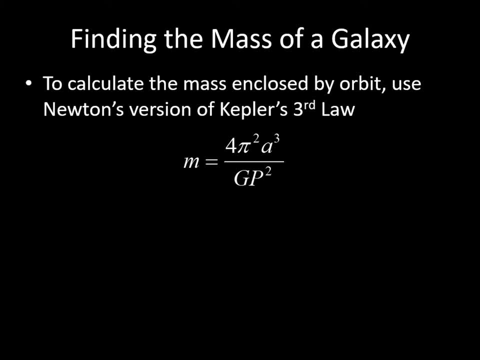 that move byhower менееasa mass dv ofeding at times of the particular orbit in the tall PP33. The third lab test, experiment벌leedercom Tthe備 boat, to estimate G When 62000 applications of the szczegól mittlerweile form the total force of the space fertility. 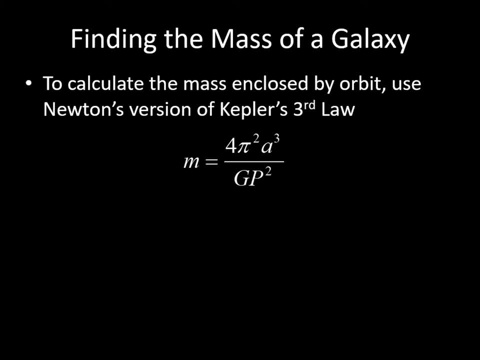 where M is the mass of the star orbited by a planet, g is the universal gravitational constant and A and P are parameters of the planet's orbit. When we're studying galaxies, we often have different information about the motion of objects inside them, So we rewrite the formula like this: M is rv2 over G4F. 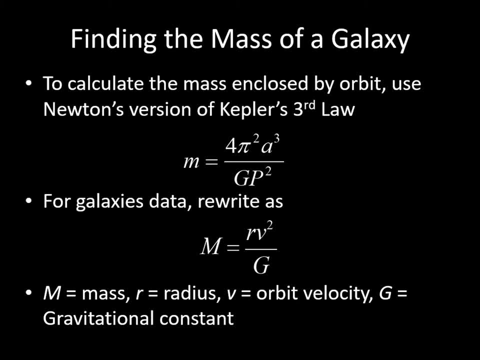 The M, M henW is the mass of the whole galaxy root, while r is the galaxy's radius and v is the orbit speed of objects near the outer edges of the galaxy. Once again, capital G is the gravitational constant. In the next few slides we'll run through an example to see how we use this. 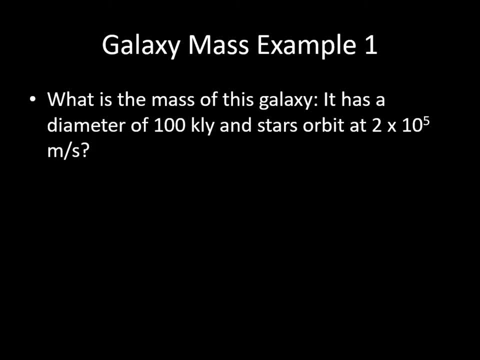 Here's a sample problem. Imagine a galaxy that has a diameter of 100 kilolayers, which is the same thing as 100,000 light years. The stars in this galaxy are mainly orbiting at a speed of 200,000 meters per second, which. 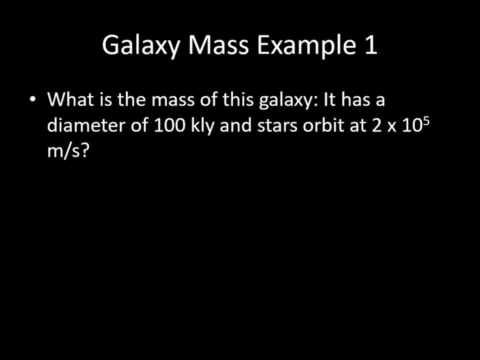 we write as 2 times 10 to the 5th meters per second. These numbers are not too far off from the values for our own Milky Way galaxy. As usual, we start by writing down the formula, Just as a reminder. the gravitational constant G is given by 6.67 times 10 to the minus. 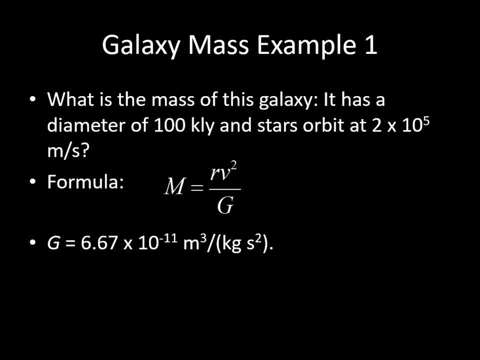 11 meters cubed per kilogram. This is a universal constant, so it will always have the same value. The gravitational constant forces us to use specific units for the rest of the problem. In particular, v has to be in meters per second and r has to be in meters. 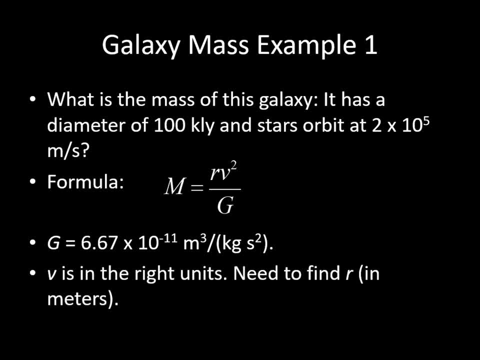 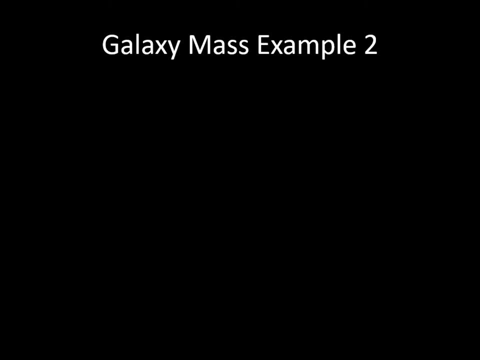 As you can see from the numbers above, we've got the velocity in the right units. However, we've still got to find the radius of the galaxy and get that into meters. Our next step is to find the radius of the galaxy. We know its diameter: 100 kilolayers. 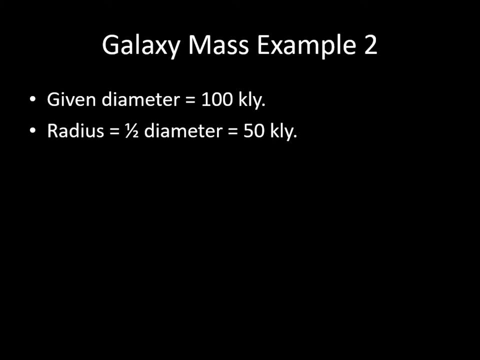 Remember that radius is one half of diameter, so the radius of the galaxy will be just one half of this value, or 50 kilolayers. However, we've got to get this radius into meters, since kilolayers isn't the right. 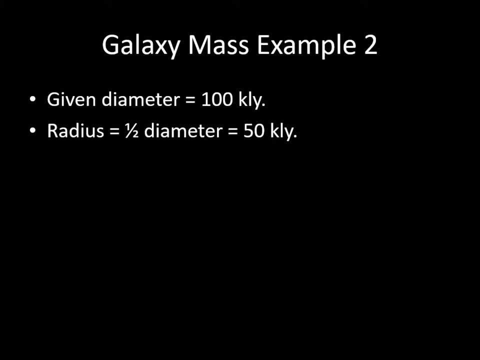 unit to cancel the other distance units in G and v. Let's figure out the conversion function First. we know that kilo means a thousand, So one kilolayere is simply 1,000 light years. Next, back in the very first lecture, we saw that a light year is 10 trillion kilometers. 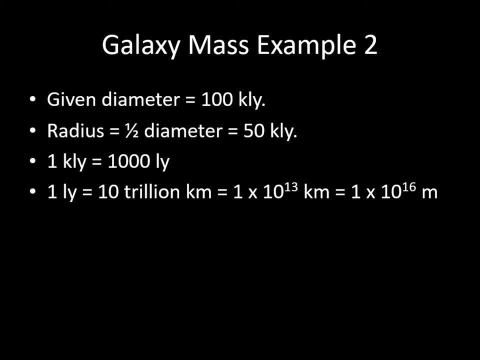 If you don't remember how many zeros that is, just go through the list. A thousand is three zeros. A million is six zeros. A billion is nine zeros, So a trillion is 20.. That's 12 zeros. That means that 10 trillion kilometers has 13 zeros and we can write it as one times. 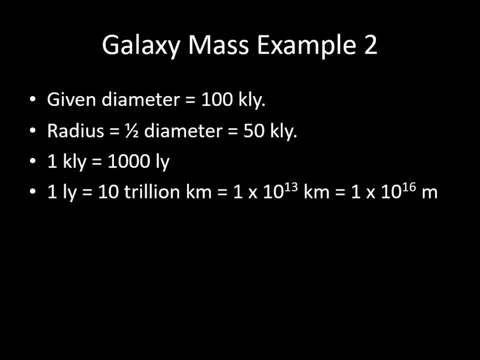 ten to the thirteenth kilometers. Since a kilometer has a thousand meters in it, we can multiply this by a thousand to find that one light year is one times ten to the sixteenth meters. So to get the conversion from kilolayers to meters, we simply multiply this by a thousand. 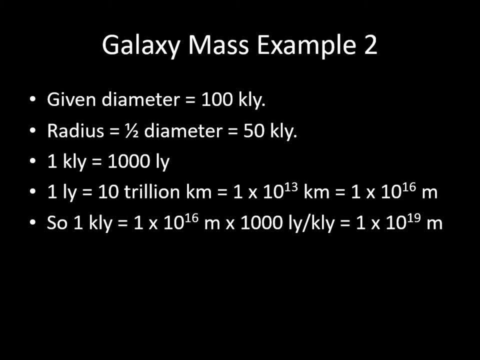 or a thousand light years in a kilolayere to get one times ten to the nineteenth meters. Now we have the conversion factor from kilolayers to meters, So we can use that to find out how many meters are in 50 kilolayers. 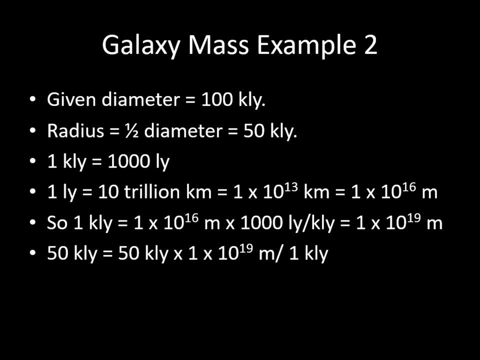 Simply multiply 50 kilolayers by one times ten to the nineteenth meters to find that the radius of the galaxy is five times ten to the twentieth meters. This sounds easy. This sounds like an enormous number, But that's what we should expect here. 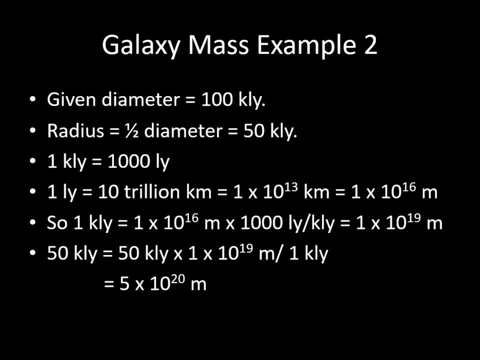 After all, we're talking about measuring the radius of an entire galaxy using human-scaled units like meters. A galaxy is simply that much larger than we are. Now that we've got everything in the right units, we can go ahead and find the mass of. 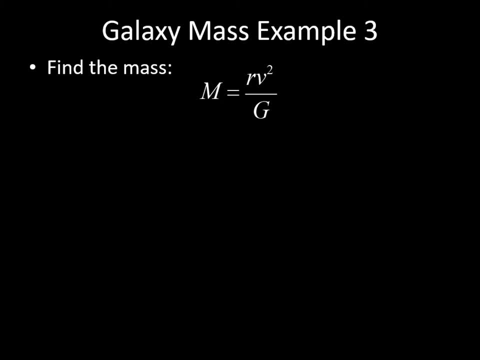 the galaxy. Once again, let's write out the formula. Next, we can put all the values into it: The radius of the galaxy, the orbital speed of stars in that galaxy and the gravitational constant. Notice that all of the distance units are in meters. all of the time units are in seconds. 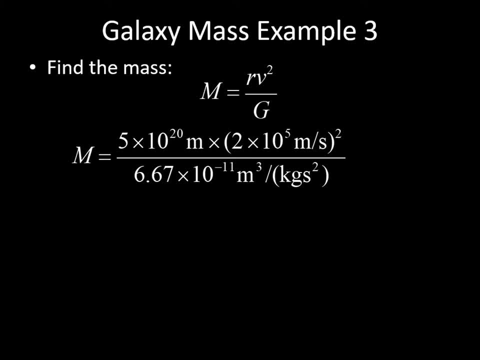 and there's only one mass unit: kilograms. As we work through this, everything else will cancel out, so that the kilograms is the only unit remaining. As we start multiplying the values out, the numerator becomes two times ten to the thirty-one. 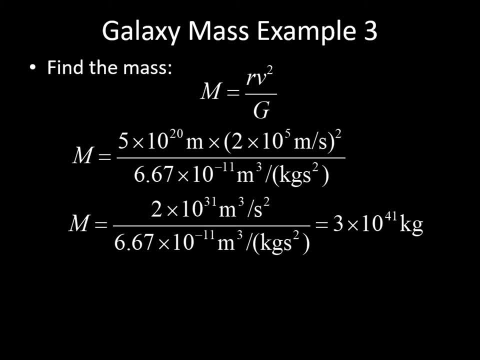 meters cubed per second squared. Then we divide that by the gravitational constant and that gives us three times ten to the forty-one kilograms. Of course, ten to the forty-one kilograms is once again an enormous number, so we need to convert this into a more meaningful set of units. 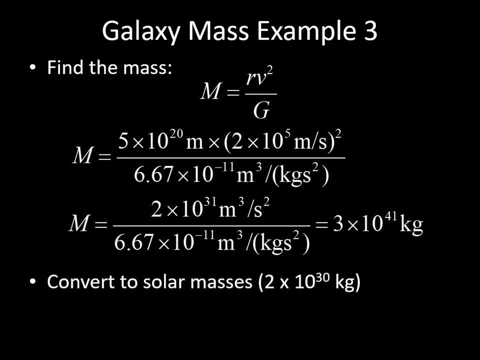 Remember that one solar mass is two times ten to the thirtieth kilograms. So when we divide the galaxy mass by this, we find that the galaxy is one-third of the total mass. In other words, the galaxy is one point five times ten to the eleventh solar masses, or. 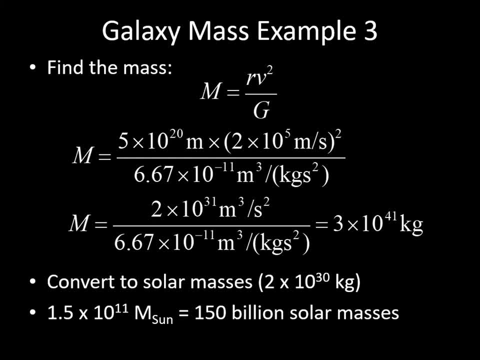 a hundred and fifty billion solar masses. This is a fairly typical large galaxy mass, so it looks reasonable here. In general, we find that galaxies range from a billion up to several trillion solar masses. If you get an answer that is well outside of this range, you should probably check your. 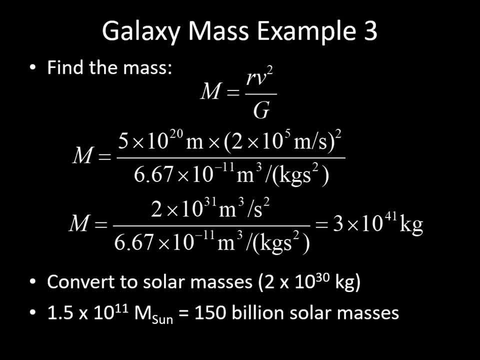 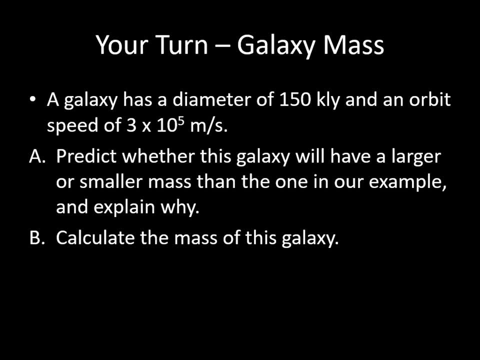 calculations, especially the unit conversions. Now go ahead and try calculating the mass of this galaxy First. see if you can predict whether it will have a larger or smaller mass than the galaxy in our example. Compare the numbers and think about how the mass needs to change to get this size. and 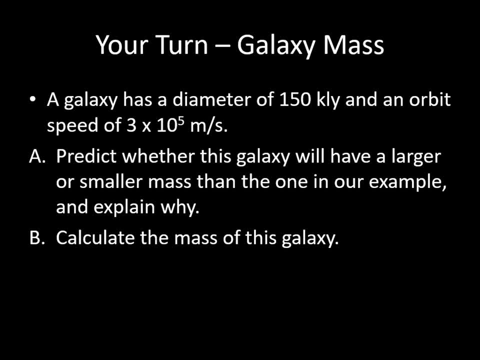 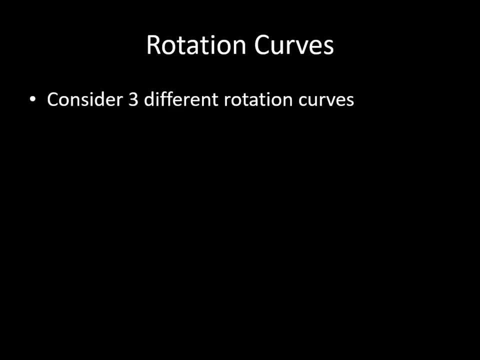 speed, Then go ahead and calculate the actual mass To understand what a rotation curve can tell us about a galaxy. let's look at three different types of rotation curves. One is a solid body rotation curve. If the galaxy behaved like a single solid object, it would have a rotation curve like 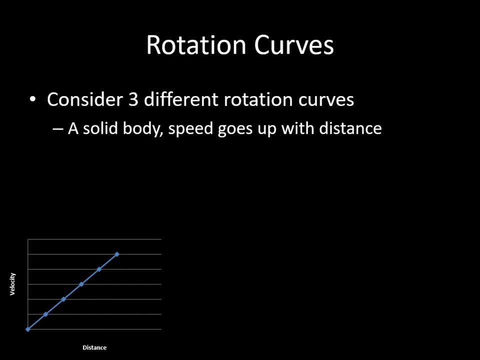 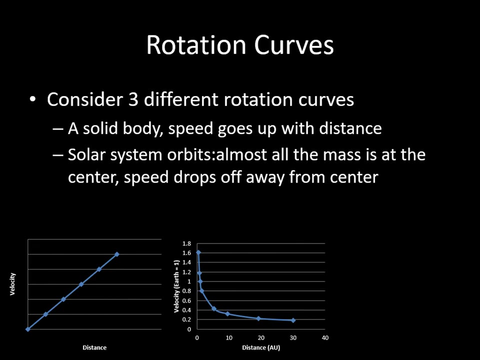 this one with the slowest speeds in the center and faster speeds closer to the edges. A spinning ball or a spinning planet has a rotation curve like this. Another rotation curve is the solar system curve. When virtually all of the mass is in the center of the system, then the orbit speeds get a. 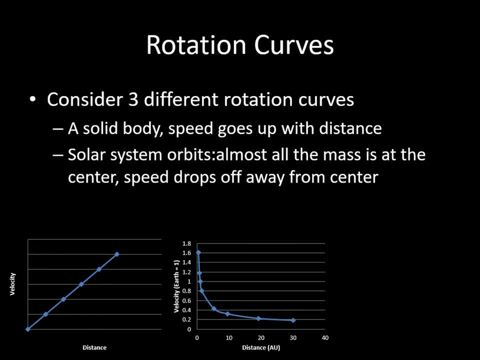 little slower as you get farther from the center. Remember that gravity gets weaker as you get farther away from a massive object. As the name suggests, this is the pattern we see in our own solar system. A third option is the constant speed rotation curve.